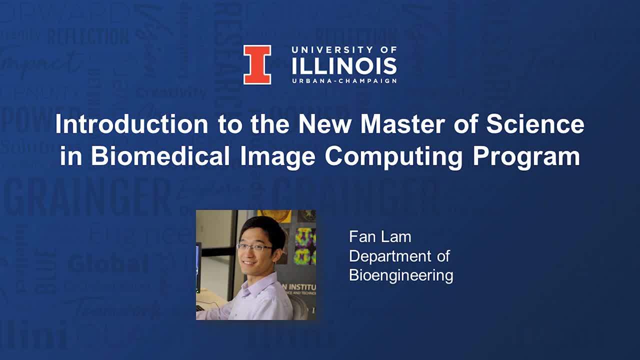 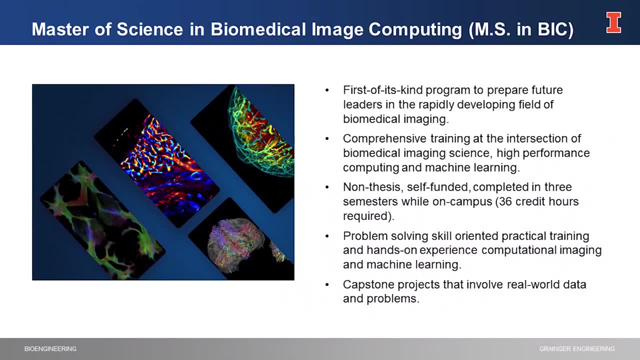 And it's really a great pleasure today to give some brief introduction to you about this very exciting program that we are building And just some context. so our vision to create this MSBIC program is really to actually establish the first of its kind of a program in the country to actually 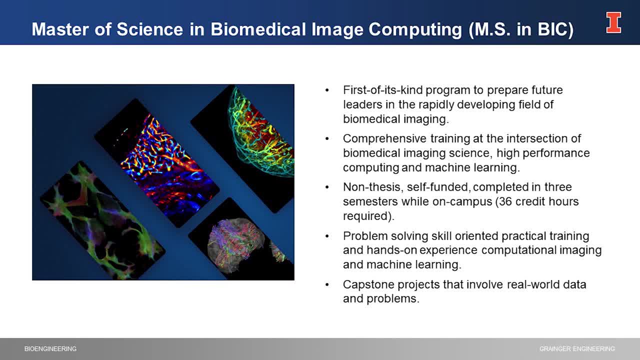 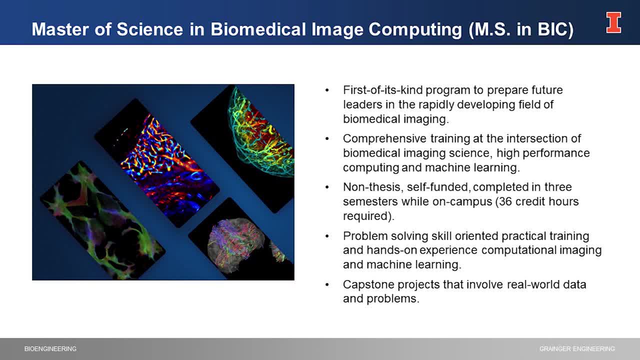 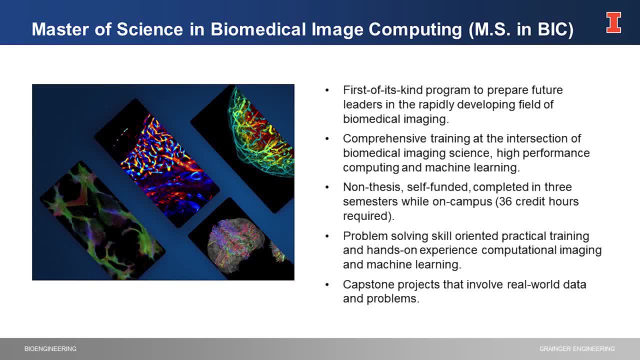 on the left here. they are all produced by technologies developed by our colleagues on this campus. I really offer you unprecedented views, tools to actually allow us to visualize, understand and quantify biological processes and physiological processes in our body. And in the meantime, we also notice this trend of this rapid development of machine learning. 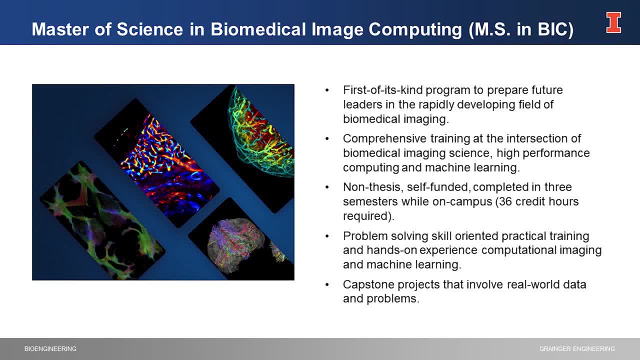 and particularly deep learning and artificial intelligence. high performance computing in the past few years is really transforming the field of biomedical imaging as we know it, And I believe it will continue to do so in the coming years. And again, coming back to these images, they are actually all produced using technologies. 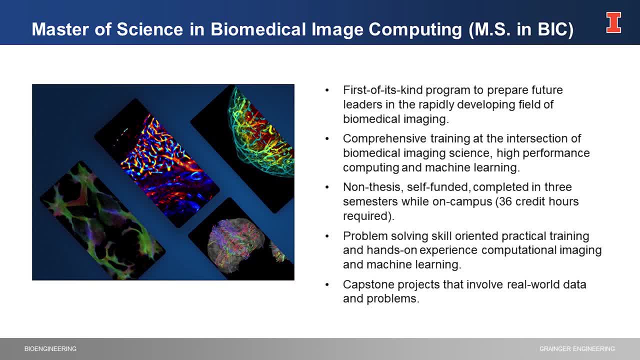 that highly synergistically integrating not just imaging instrumentation- state-of-the-art imaging instrumentation- but also highly sophisticated computational methodologies and machine learning methods. And we really want to provide, in this context, a new type of training, comprehensive and rigorous training at this unique intersection of biomedical imaging, high performance computing and machine learning. 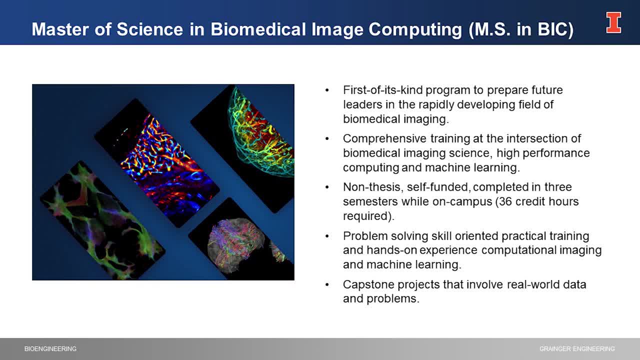 And this is a non-thesis, self-funded, three-semester, pretty intense program And right now we only offer on-campus option, but we are definitely looking into the possibility of doing an online version as well, And we really emphasize on training the student. 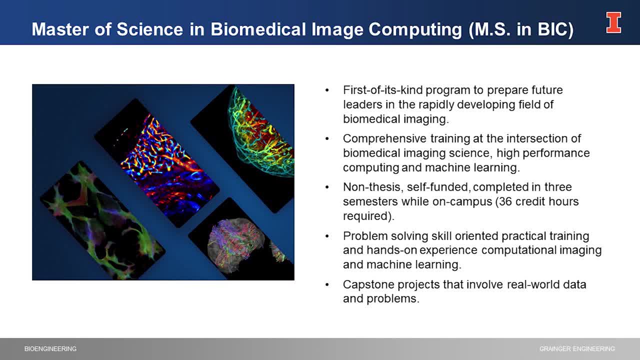 to make sure they have a good, solid understanding of the tool- the machine learning AI tools that is being rapidly developing these days, and also develop practical skill set to allow us to formulate machine learning AI solutions to practical and challenging biomedical problems. And then we also offer capstone project. 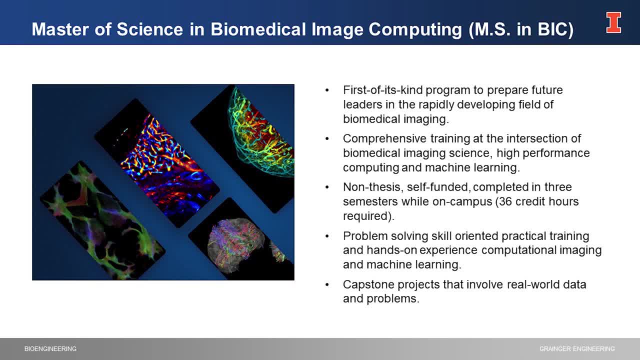 during which you will have the unique opportunity to work with world-leading experts in biomedical imaging across the campus and also from industrial partners. We'll talk a little bit later. when you look at the curriculum And based on our research and the demand from the job market is robustly increasing. 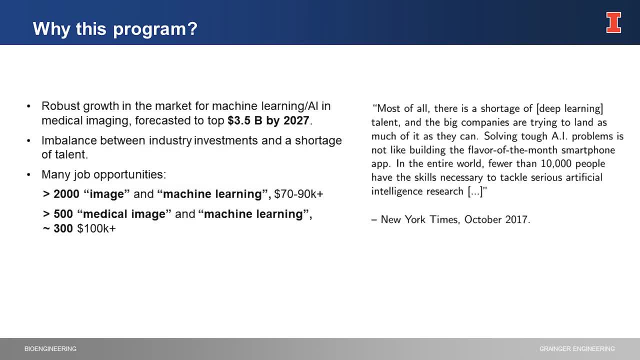 and just to give you some numbers, it is expected to see a very robust growth in the market for machine learning AI and the industry of machine learning AI in medical imaging, And it's four countries forecasted to top more than three billion dollars as a trillion a billion dollar industry by 2027. 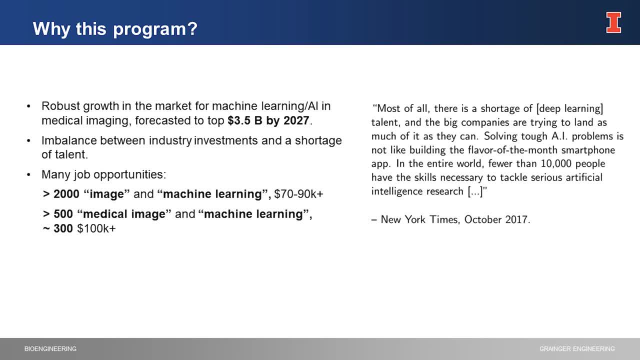 And, more importantly, I want to emphasize that this really strong imbalance between the demand from industry, research institution as well as the government agency, in the skill set and talents in biomedical image and biomedical data science, and the imbalance between this demand and then the shortage of supply. And to highlight this imbalance, I would like to read this quote from: 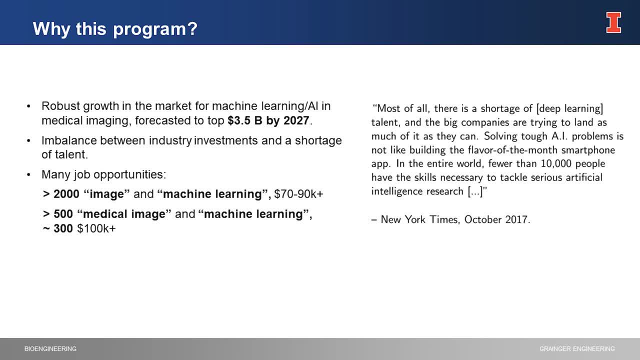 New York Times from 2007 and it says that there's a real shortage of deep learning talents and the big companies are trying to learn as much as often as they can. solving tough AI problem is not like building flavor of the smartphone app. in the entire world, Fewer than 10,000. 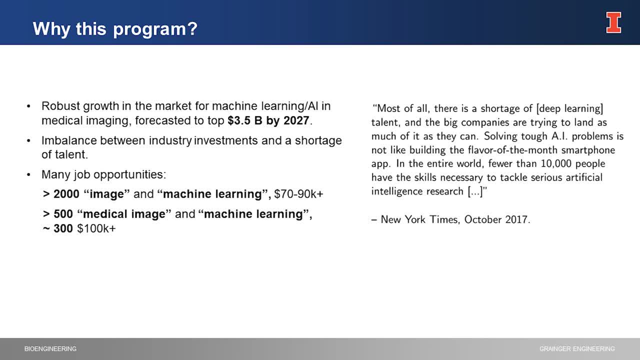 people have the skill necessary to tackle serious artificial intelligence research. So you can be one of these people. if you get our program And some additional numbers, And if you do a quick search on JobBall like Indeed, you will easily find more than 2,000. 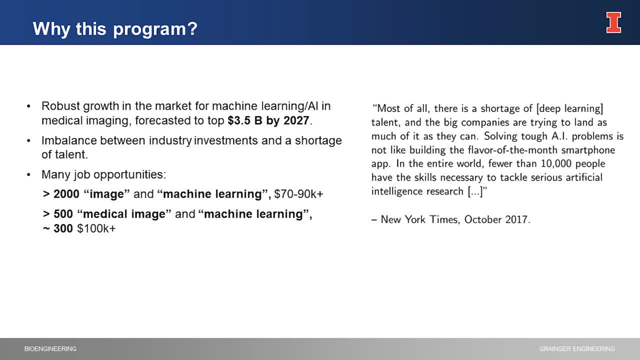 jobs in using keywords like image and machine learning, And more than 1,500 of them has an expected salary of 90K. Now that money is so important, And if you reduce the term, if you reduce the search to medical image and 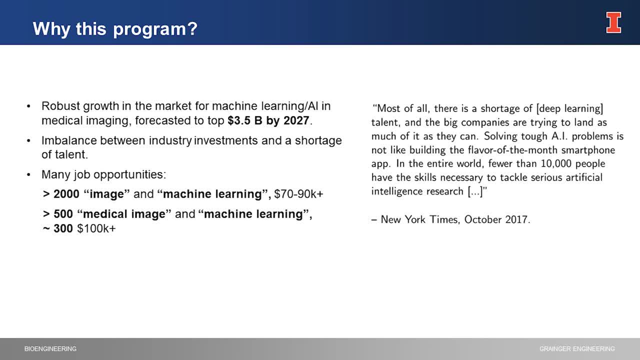 machine learning you will also find more than 500 of them, And then about 300 of them has an expected salary more than 100K. So this is actually from a year ago, So it will be interesting to see what the number has changed. 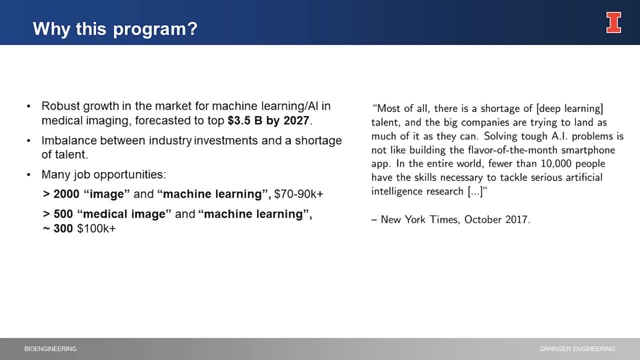 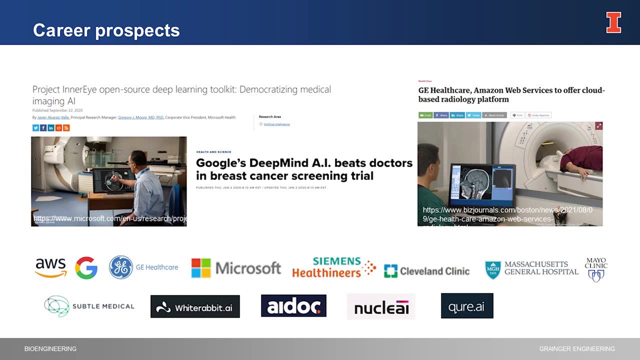 over the past year or so. And then- one nice thing about this, as we're looking into this- a lot of job opportunities offer remote working flexibility, So you don't have to travel a lot, Okay, And the career process is quite exciting. 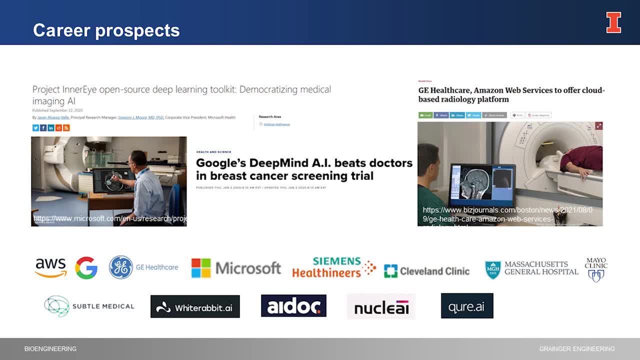 In fact, the more I look into this, the more I wanted to enroll in this program myself. So if you pay attention to the news these days- not the fake ones- you will notice that many of these big tech giants are really heavily invested. 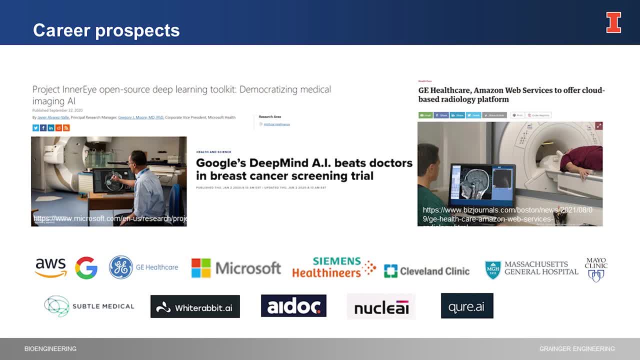 in this general area of AI and healthcare, And a very major component of this area is to develop AI-based software or algorithms that can automatically detect, diagnose and characterize disease and also support clinical decision-making process. You will notice that there are a lot of. 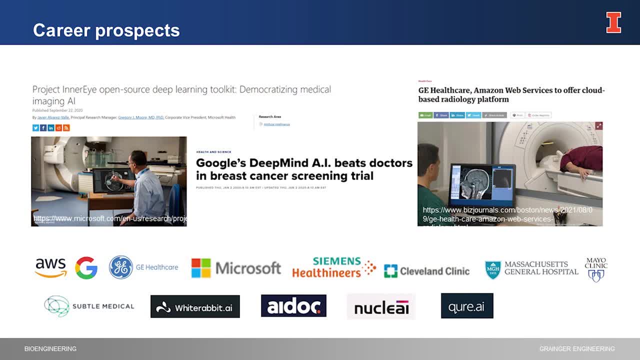 big tech companies using the large volume of imaging data that we routinely collect from individual patients these days And then potentially integrated with other clinical data, such as genomic data. So we have this sheer very, very huge volume of data from individual patients that we need advanced tools and algorithms. 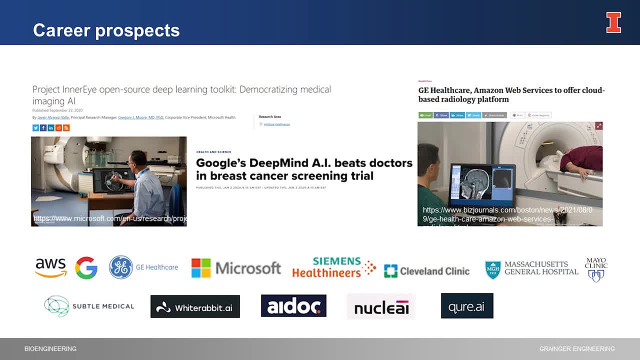 to help us make clinical decisions with, And so there are really a lot of opportunity in not just in big tech companies, but also in big tech companies, right, And that is really looking for people to have the skill set in biomedical imaging, biomedical imaging analysis. 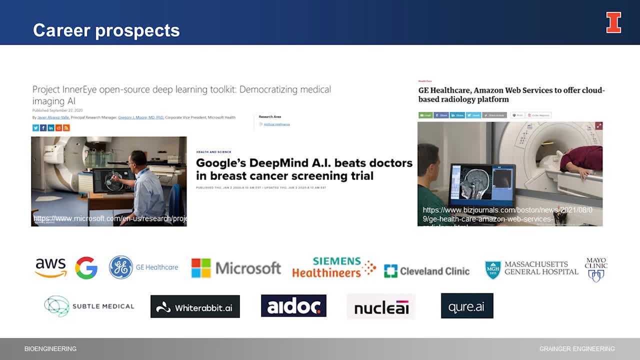 and biomedical data analysis. But there's also a unique opportunity from major healthcare providers and research hospitals, major hospital systems in our country, because of this unique space of biomedical imaging computing. It's really a synergy between machine learning, high-performance computing and biomedical problems. 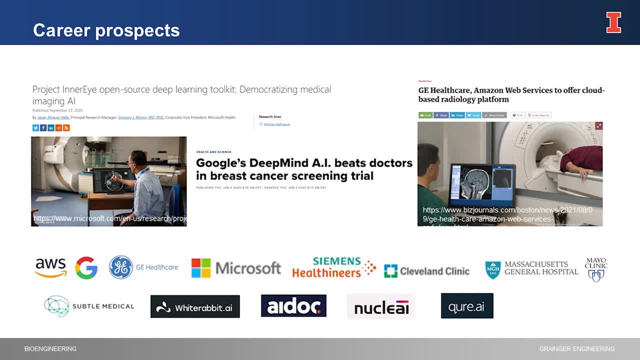 And also we know we notice this very apparent trend in the past few years is that this is really increasing number of start-up companies that are showing up across the world. try to focus on developing AI-based software to make intelligent clinical decision-making, to support biomedical image and biomedical data analysis. 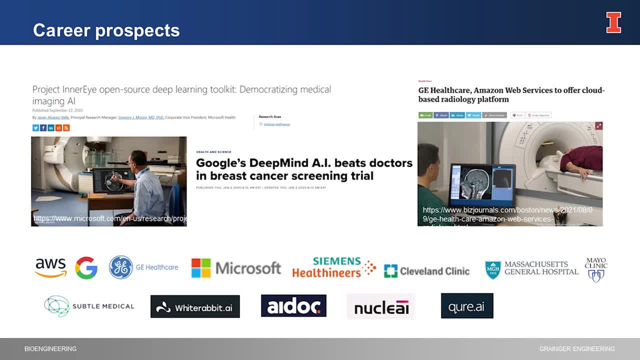 And if you know, this biggest society of radiology, this country called RSNA, they have this annual meeting to RSNA And then if you go to the meeting five years ago, so you don't see many AI companies, But if you went to the meeting 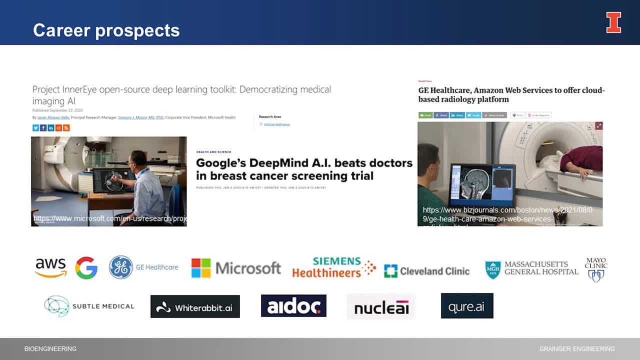 a couple of years back, you will notice that suddenly there's this dedicated hall, exhibition hall, totally dedicated for companies working in the space of AI, in the intersection of AI and radiology, And there are big companies, small companies and many, many of them. 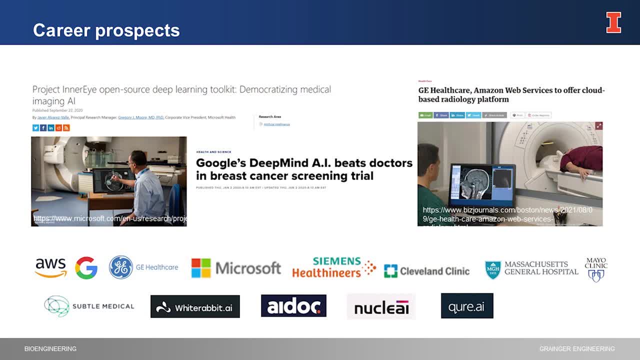 I was truly amazed when I went there, because I didn't notice this at all before. So it's a really exciting time to be in this space. And just a couple of additional examples to kind of connect to what we are talking about here. Again, you will find many opportunities. 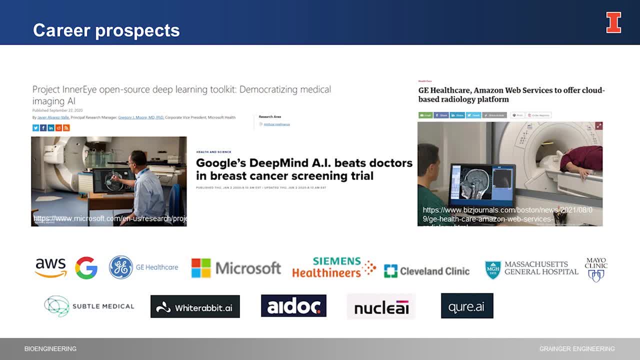 in big small tech companies, But also because of this unique space. you also find very interesting opportunities from this unique environment of the healthcare process. the provider and research, hospital systems And even insurance companies are looking for talents who can do data mining using image informatics tools. 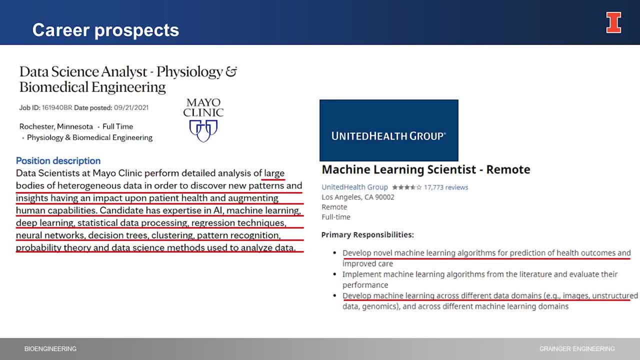 And if you read this job description, you will notice more like deep learning, statistical data processing, regression techniques, neural network, decision trees, glass screen, blah, blah blah. There's so many fancy terms here, And then this is the skill set. 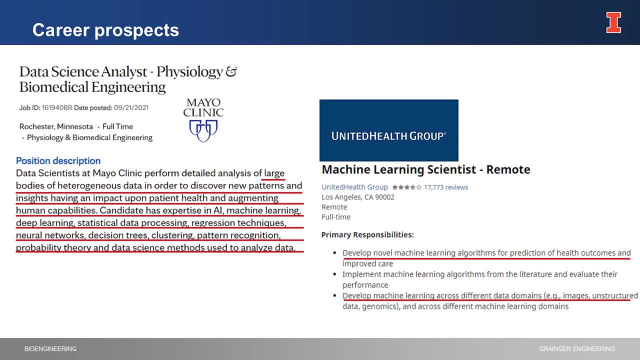 you will be equipped with when you get out of this program, And through this fairly intensive three-semester training, we go into courses that cover a very foundational biomedical imaging, science, instrumentation and high-performance computing, the machine learning, AI tools and also how to develop. 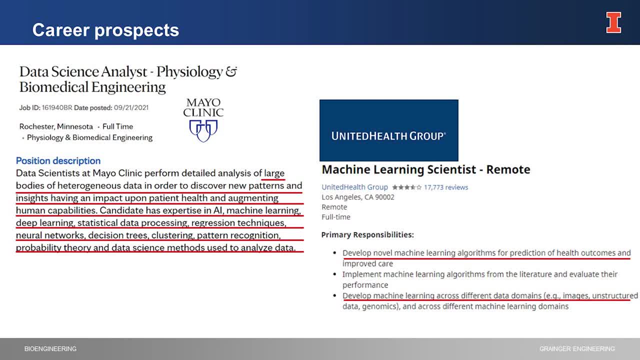 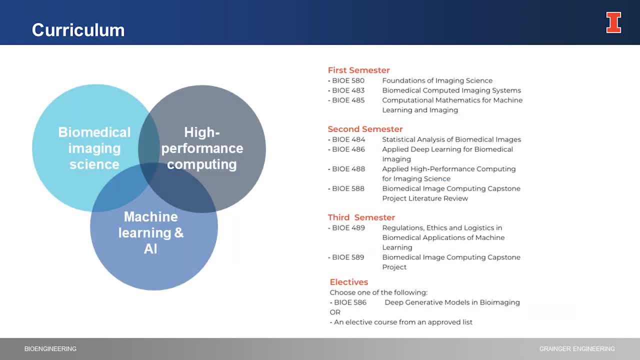 and deploy machine learning, AI solutions on high-performance computing platforms. So I won't go into the individual courses in detail, but I'm happy to. if you have more questions. I'm happy to talk about more detail about individual courses after this, And again we have capstone project. 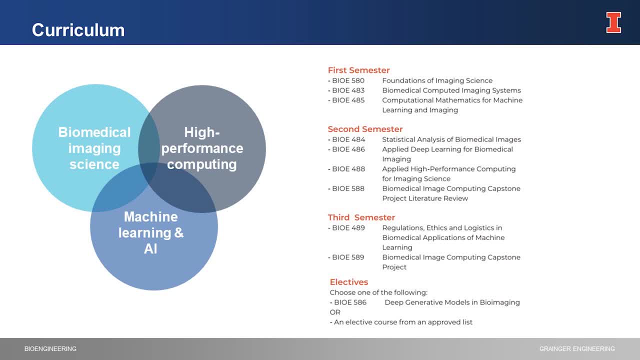 that we will design particularly to allow you to work on real biomedical imaging data and to tackle practical, real biomedical imaging problems, in collaboration with not only leading experts in this field of biomedical imaging machine learning on campus, but also industrial partners who are stakeholders in this field. 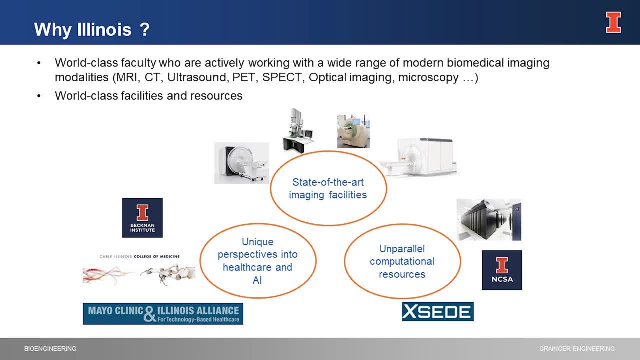 And, as I said, we really want to establish one. this is really one of the very first program that focus on this unique space in this country, And then- I will not be surprised- we will see more and more program coming out on this across the nation. 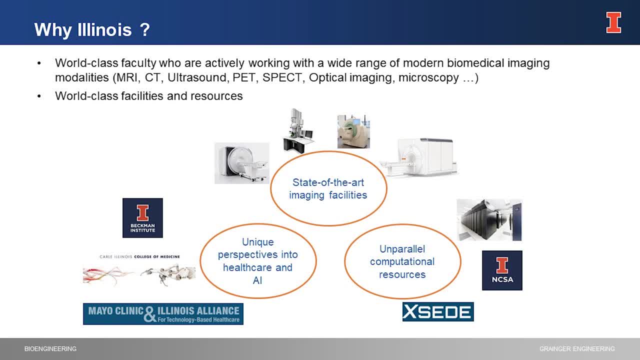 even across the globe. But I want to say that Illinois is really the perfect place for this program because we really offer a very unique resources and capacity capabilities for you to get the skillset that you would need to be very successful in this space, For example, we really have world-class faculties. 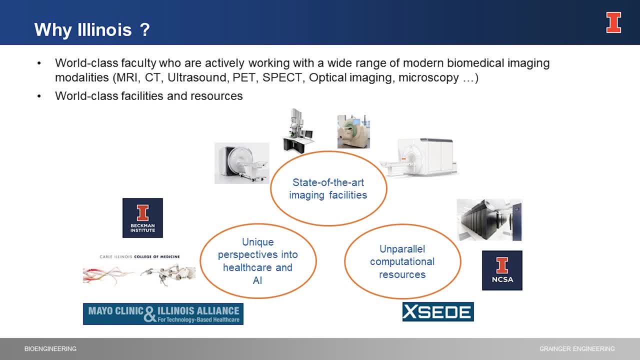 that actively working with a wide range of modern biomedical imaging modalities- MRI, CT, ultrasound, molecular imaging, optical microscopy, we name it- and we really provide a wide range of services, and I'll take a few examples and then I will wrap up. 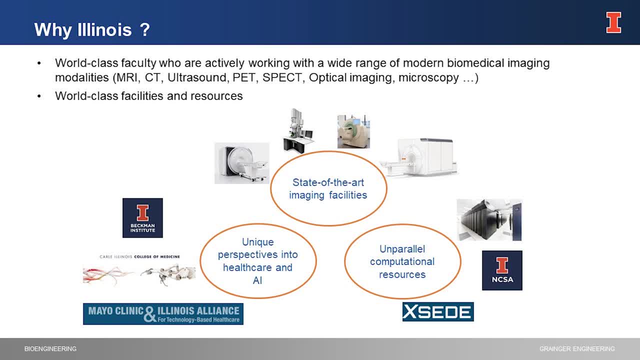 have world-class facility and resources to provide you the type of experience or training that you will want, and including state-of-the-art imaging facility- really unparalleled computational resources. we have one of the four super computing application centers of this campus- and then, because of the unique collaboration relationship between different multidisciplinary institutions. 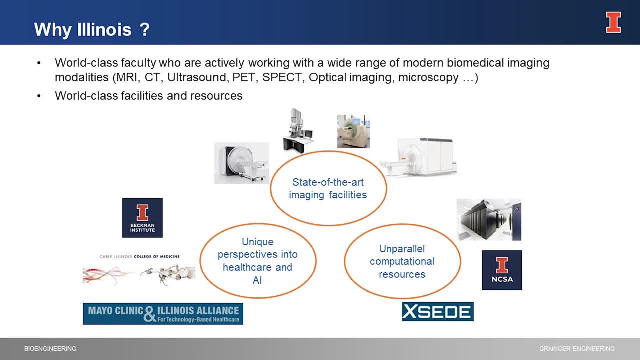 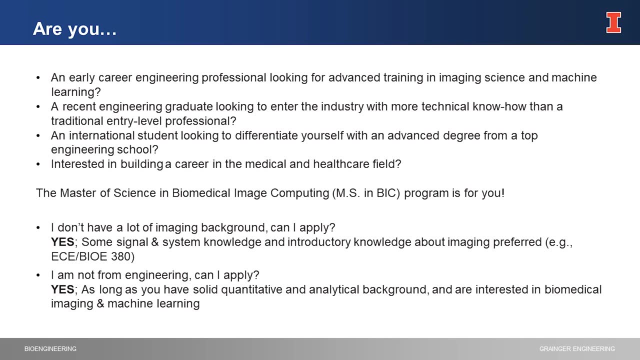 and clinical partners. i believe we can offer you the very unique expert extra perspective into the role of ai in healthcare. yeah, and then, if you are considering whether you are where this program is for you, i'm just listing out some of the factors for you to consider, but of